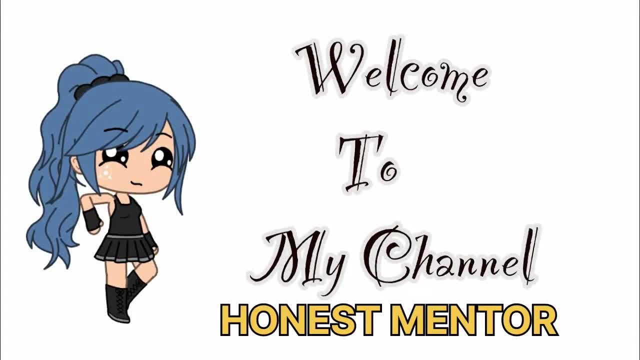 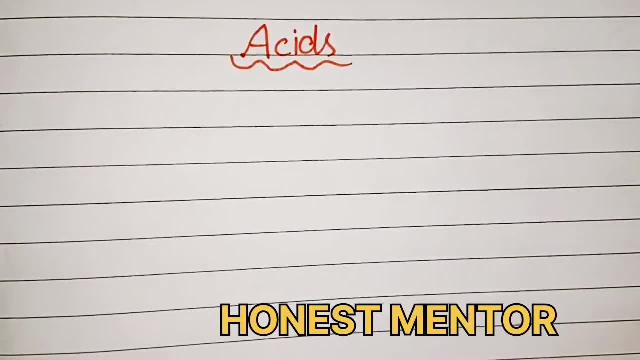 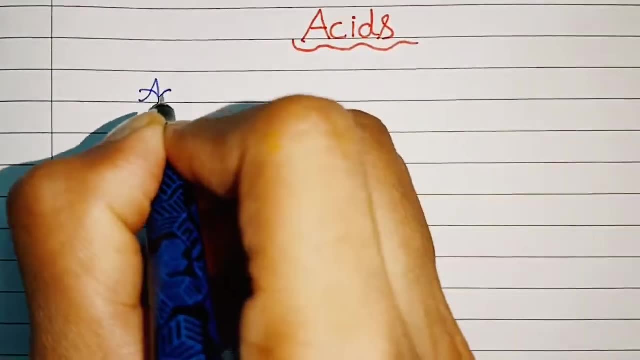 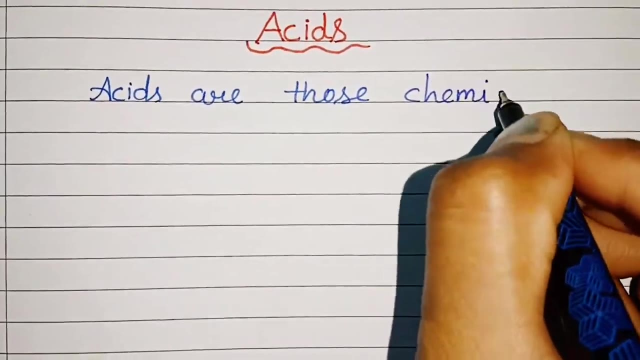 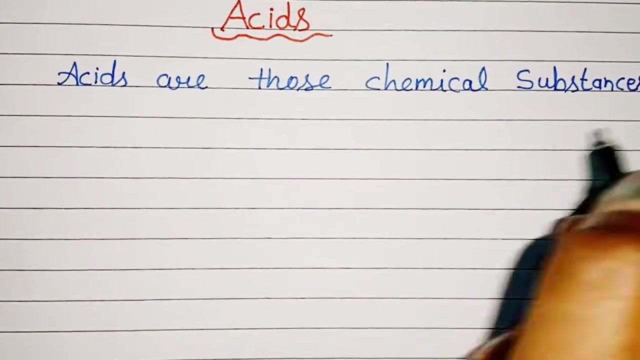 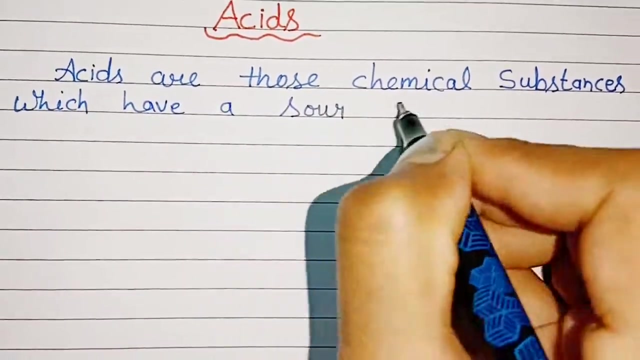 Hello everyone, welcome to my channel Honest Mentor. Today we are going to learn about acids. Let's start. Acids are those chemical substances which have a sour taste and change the taste of the food. 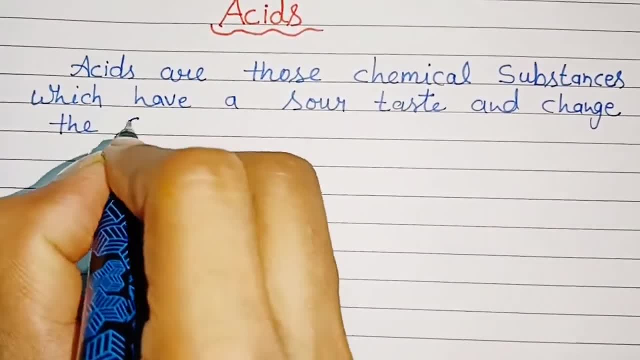 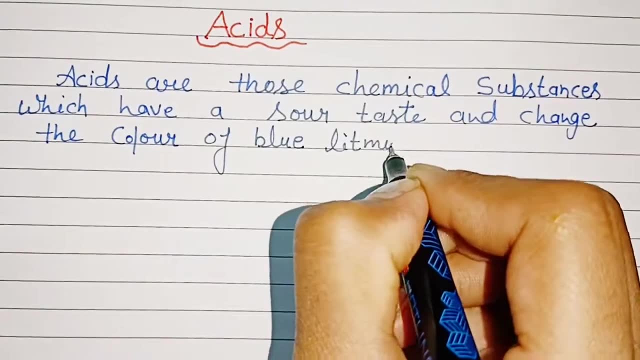 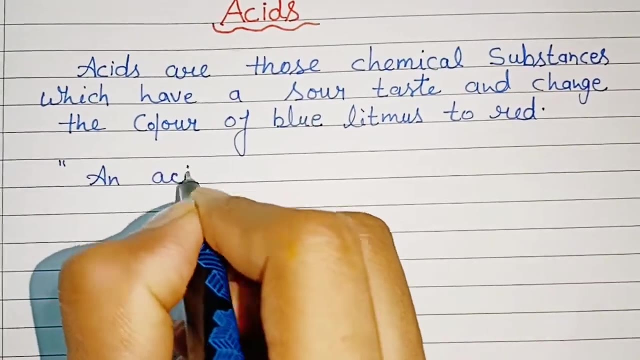 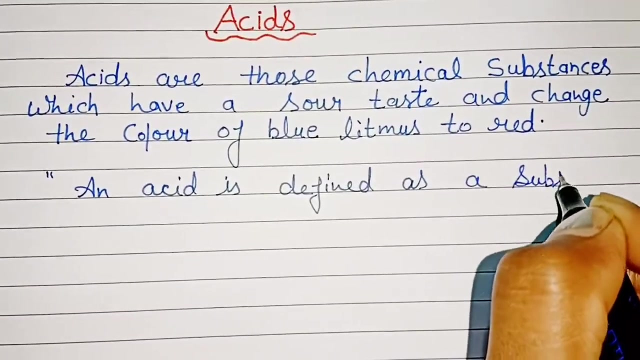 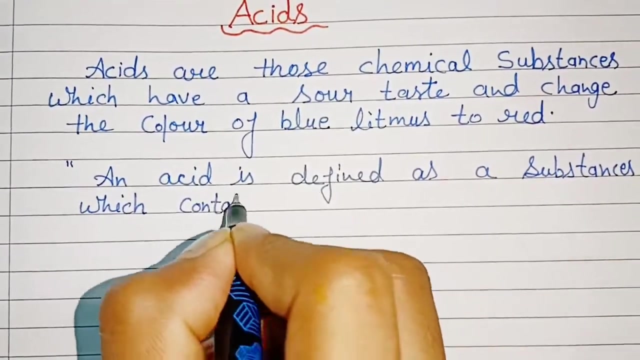 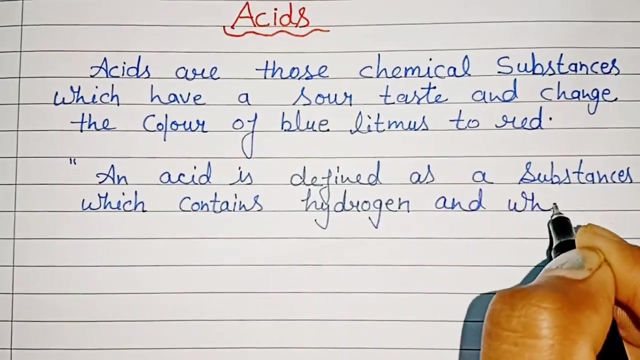 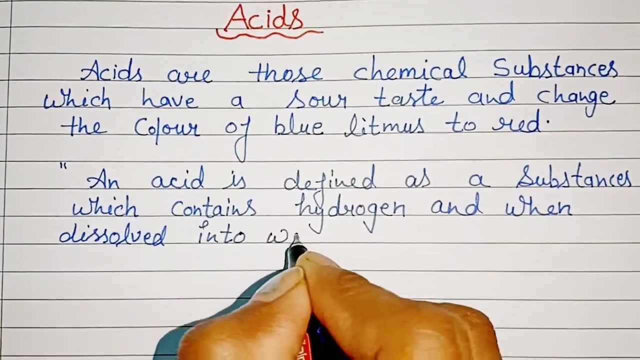 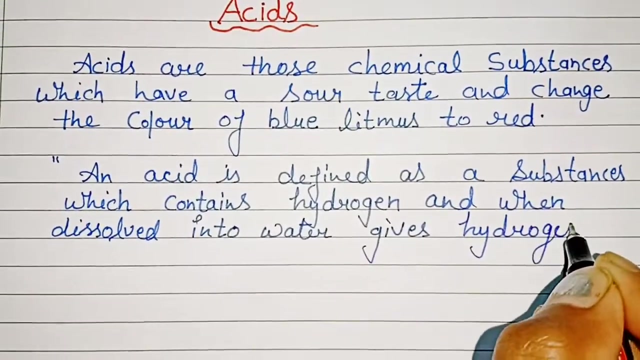 They change the color of blue litmus to red. Second definition is an acid is defined as a substance which contains hydrogen and van dissolved into water, which gives hydrogen ions H+. 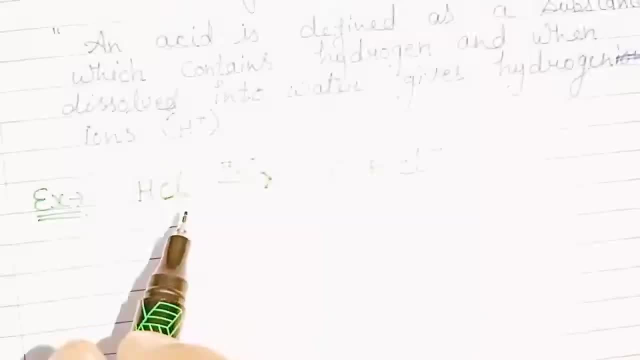 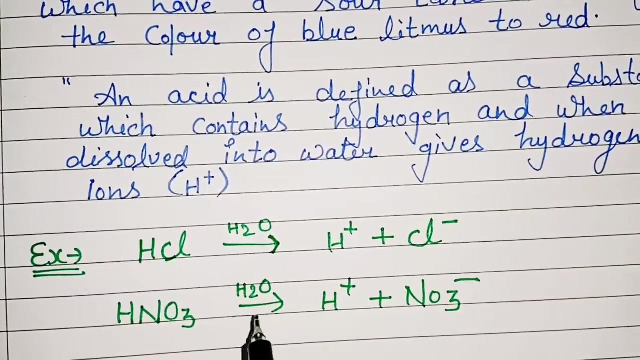 Some examples. First definition of sal water. First definition of sal water. Basically, sal water contains H+, Cl- ions HNO3 arrow S2O H plus ions N3 minus ions S2 SO4 eliminated 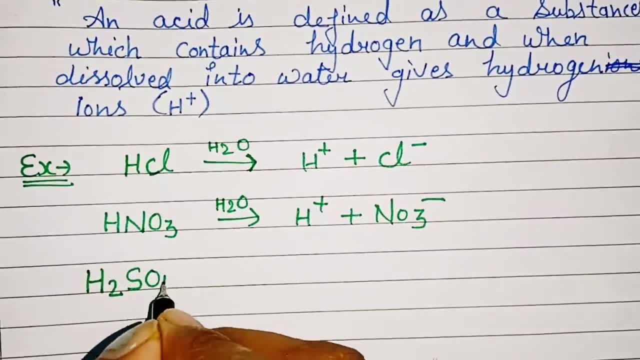 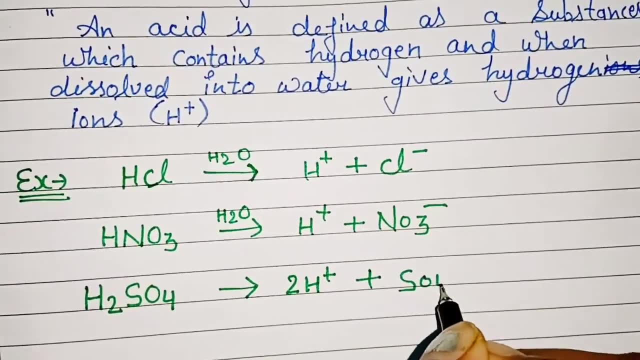 by HNO3 arrow to . Such acids are called sal water. Assessment. 2. Amino acid. 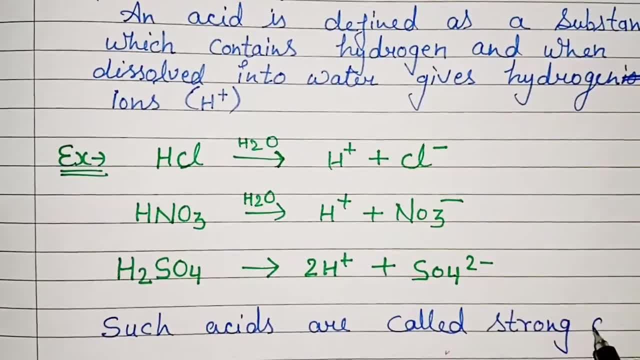 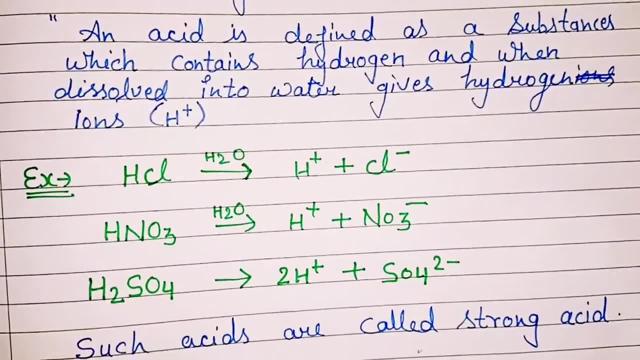 Thanks for watching my video, if you like my video don't forget to like, share, comment and subscribe also. Thanks, bye. 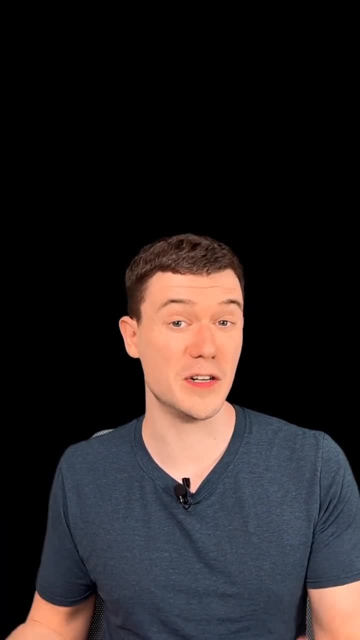 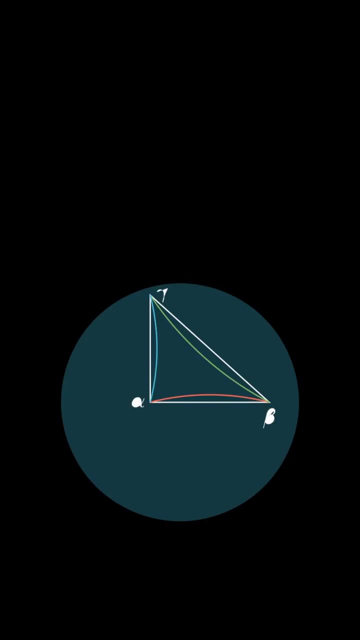 There's an even weirder non-Euclidean geometry, known as hyperbolic geometry. In this geometry- you guessed it- the angles of a triangle add up to less than 180 degrees. Here imagine triangles being drawn on hyperbolic surfaces like Pringles chips.